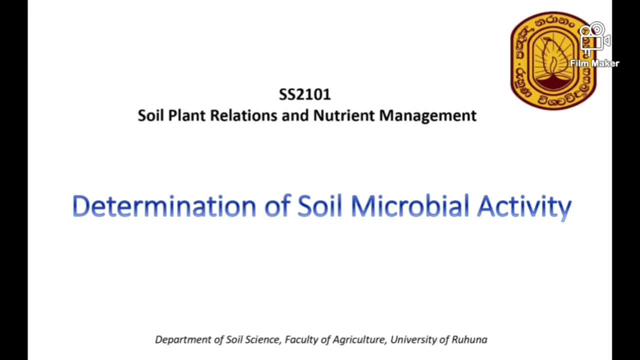 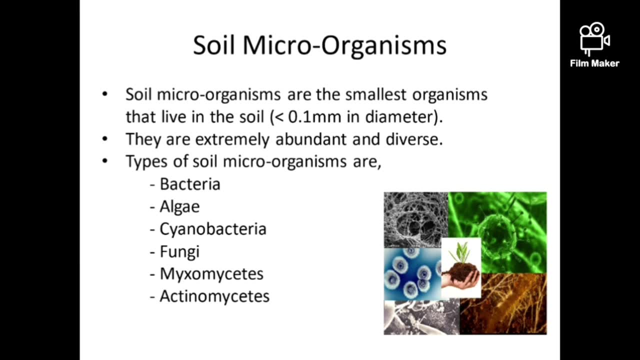 Determination of soil microbial activity. Soil microorganisms are the smallest organisms living in the soil, which are lesser than 0.1 millimeter diameter. They indicate an extreme diversity and abundance. Bacteria, fungi, algae and cyanobacteria are some of them. Rhizosphere shows the highest activities of soil microorganisms. 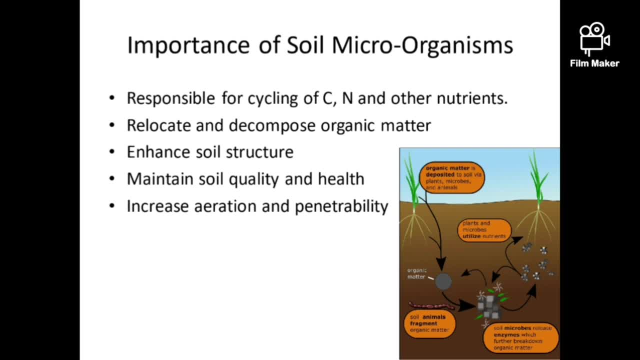 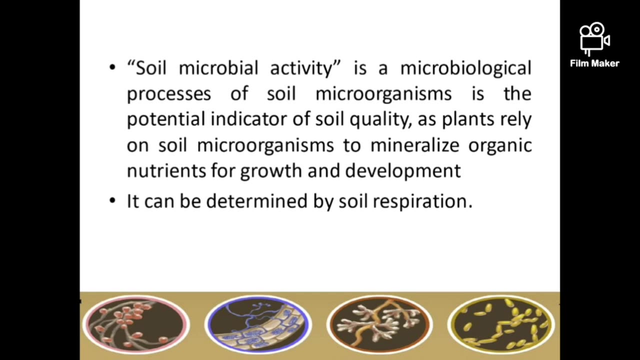 Soil microorganisms contribute to a greater variety of important and plant growth promoting activities. Few of them are mentioned in the slide. Soil microbial activity is a microbiological process of soil microorganisms. It is the potential indicator of soil quality, as plants rely on soil microorganisms to mineralize organic nutrients for good. 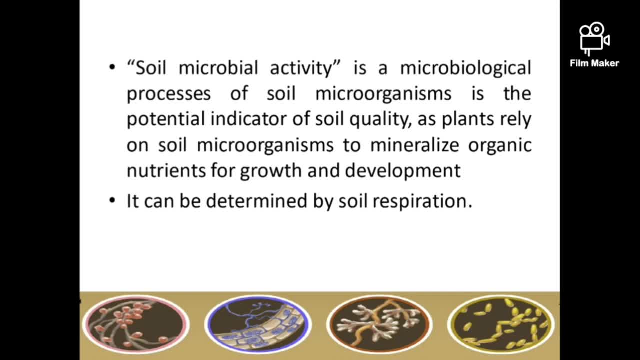 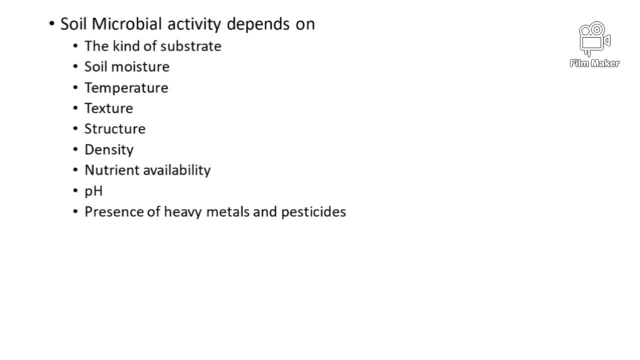 Mainly soil. microorganisms can require入격 and the right amount of fertilizer to grow and develop and get new growth. It can be determined by soil respiration. Respiration activity depends on several factors, as with type of substrate, moisture, content of soil. 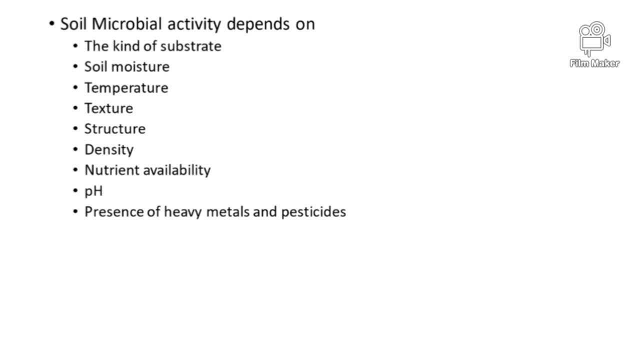 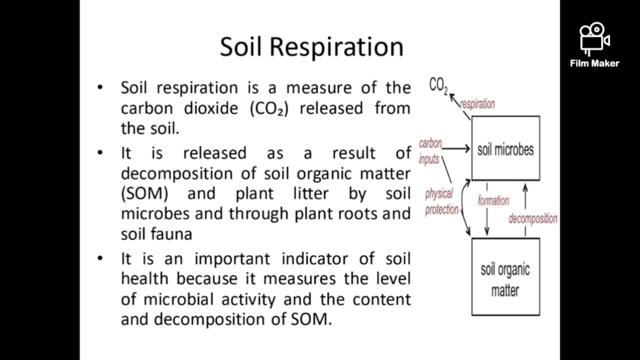 temperature, pH and so on. Evidence from thevtionfelor is that carbon dioxide released through the microbial metabolism activity Soil respiration. Soil respiration is a measure of the carbon dioxide released from the soil. It is released as a result of decomposition of. 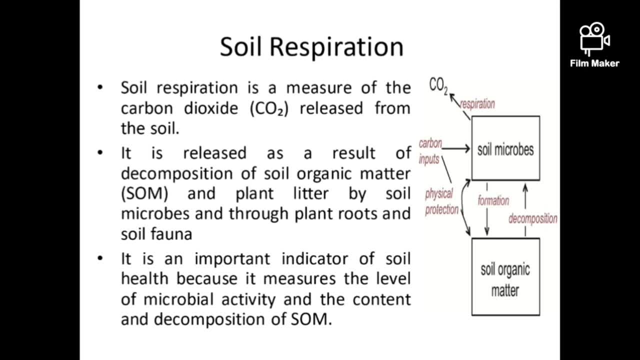 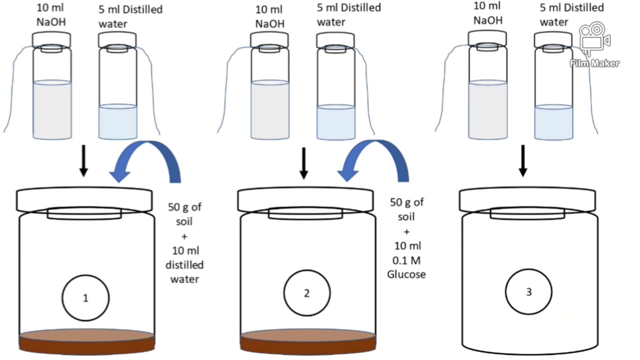 soil organic matter and plant litter by soil microbes and through plant roots and soil fauna. It is an important indicator of soil health because it measures the level of microbial activity and the content and decomposition of soil organic matter. This is the brief procedure of the practical 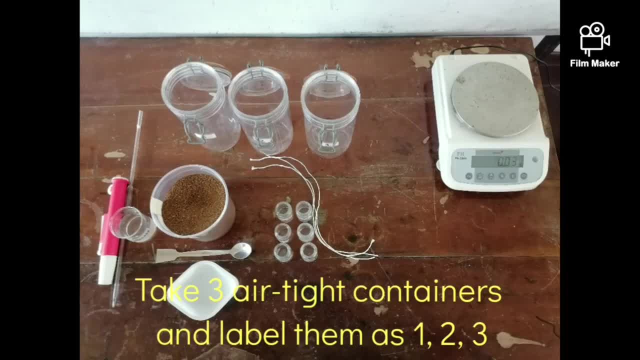 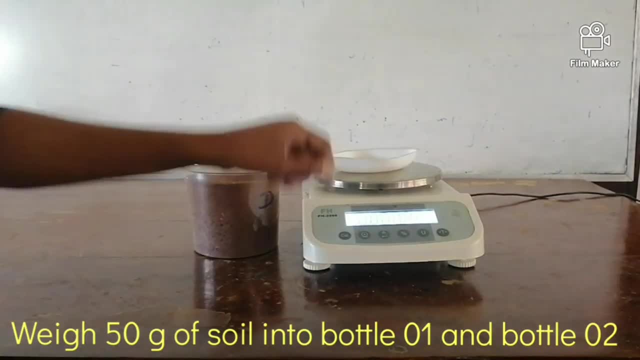 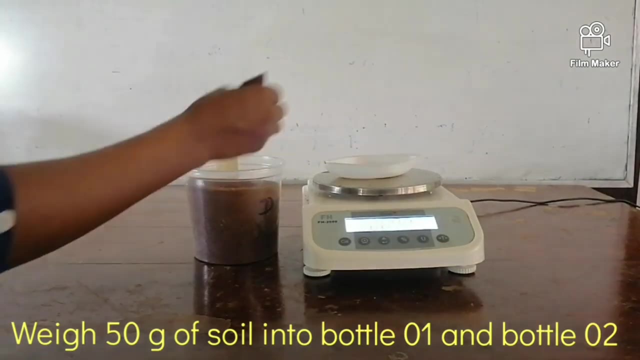 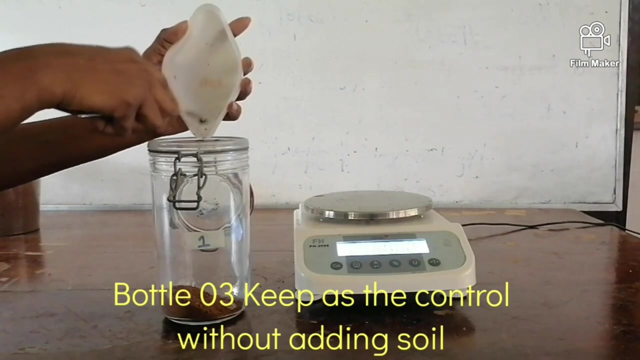 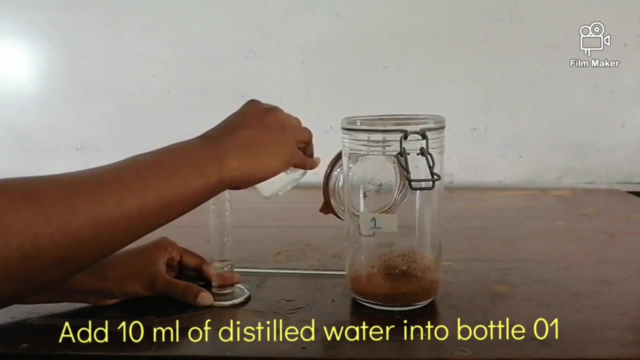 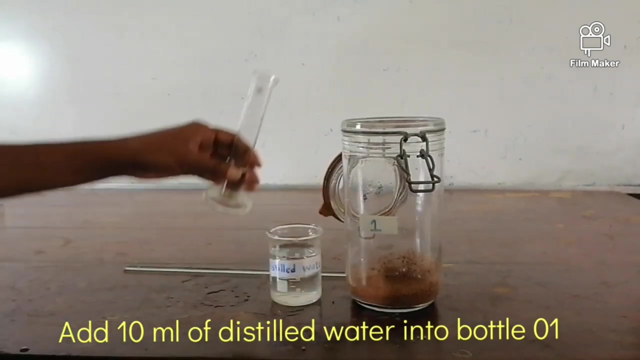 Take three airtight containers and labour this as 1, 2 and 3. You have to weigh 50 grams of soil into bottle 1 and bottle 2.. Bottle 3 keeps as the control, without adding any soil. Next, add 10 ml of distilled water into bottle 1 and mix it properly with the soil by using a glass rod. 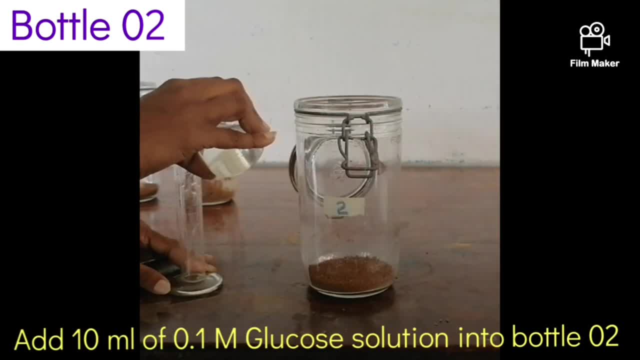 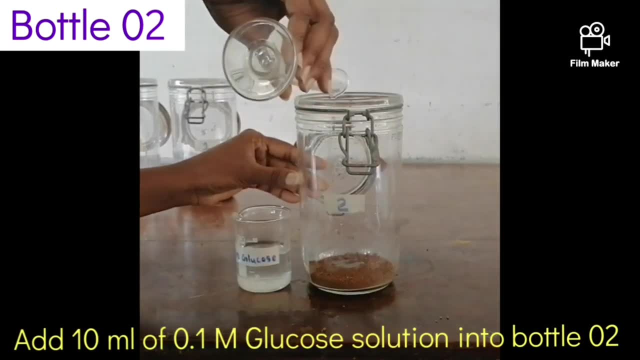 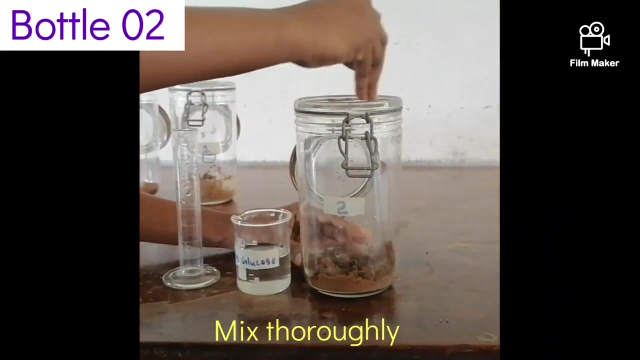 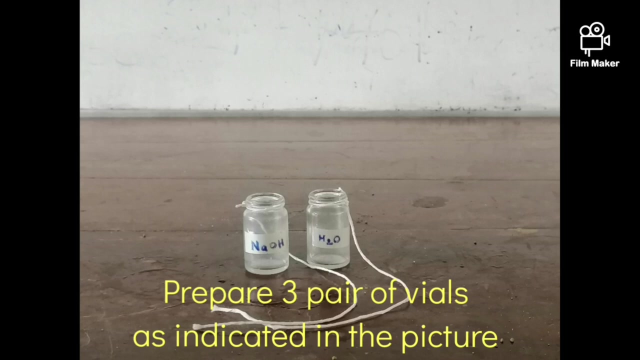 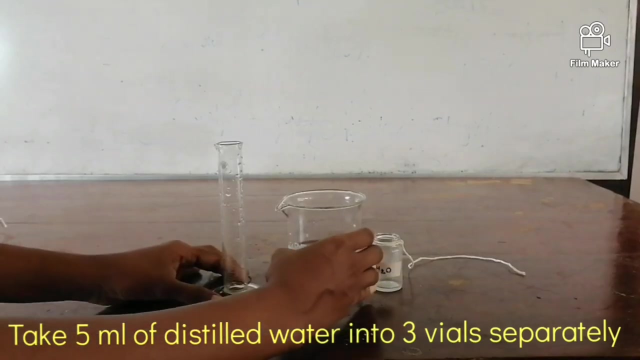 Then add 10 ml of 0.1 m glucose solution into bottle 2. And it should be also mixed well with the soil. You have to prepare 3 pair of sodium hydroxide and distilled water vials. Take 5 ml of distilled water into separate 3 vials. 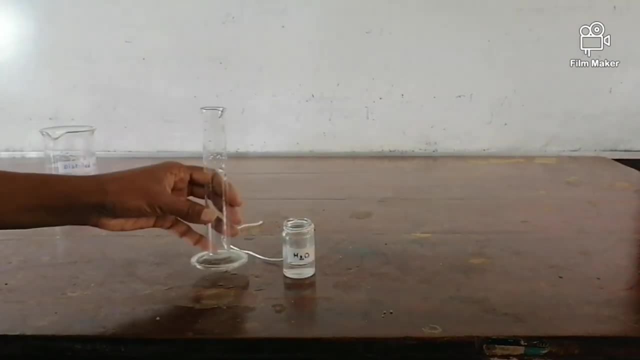 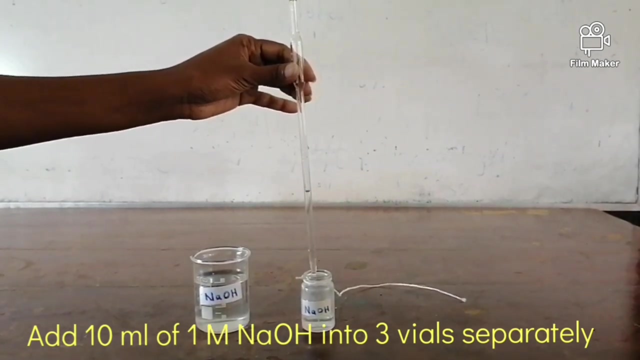 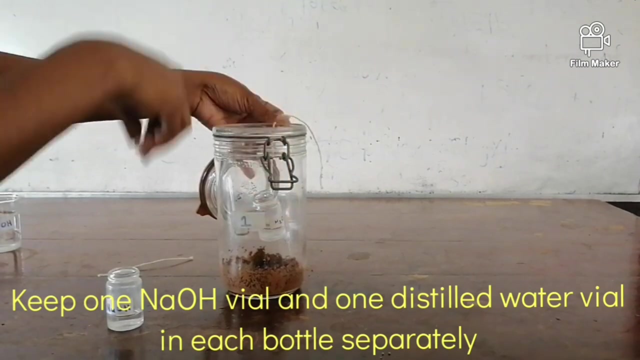 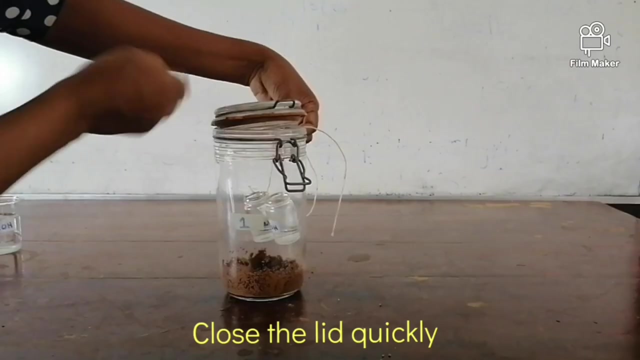 As well. measure 10 ml of 1 m sodium hydroxide and put it into separate 3 vials. Keep 1 sodium hydroxide vial and 1 distilled water vial in each bottle separately And close the lid quickly. 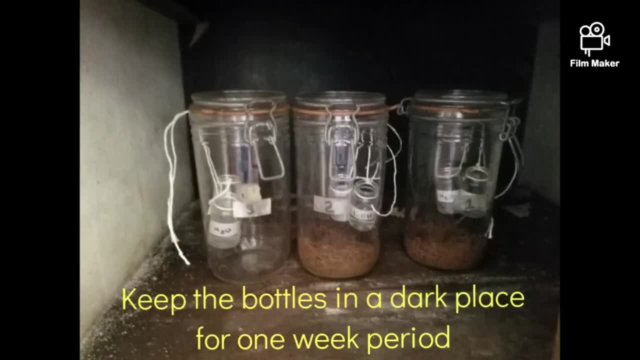 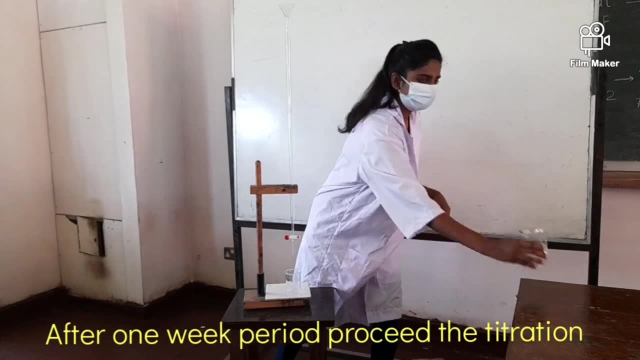 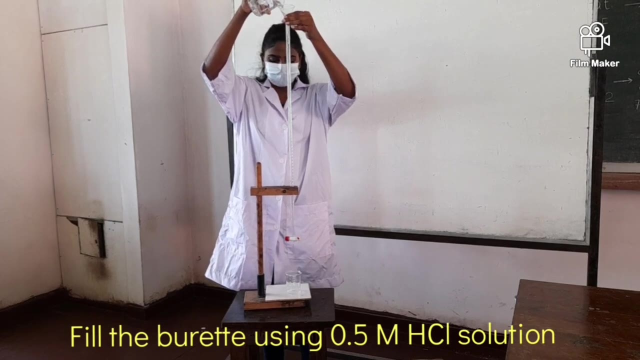 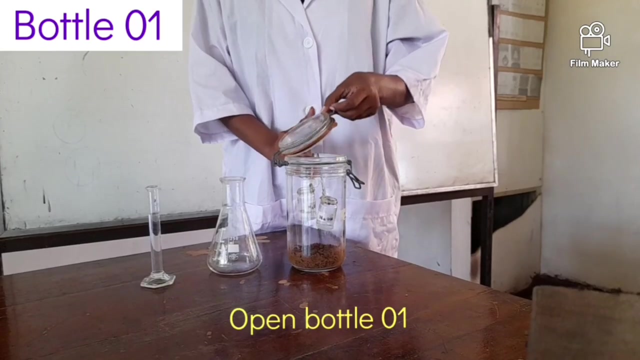 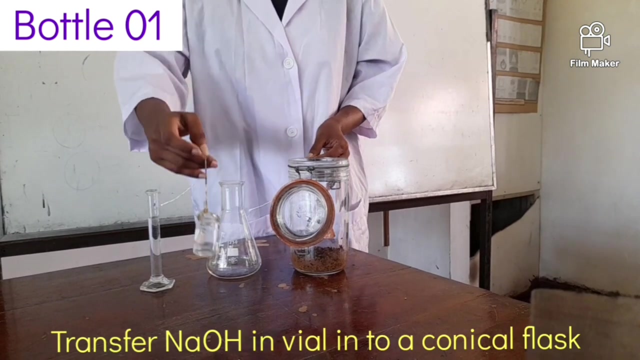 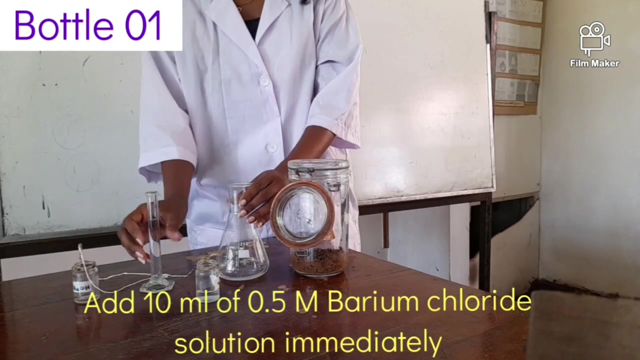 Then incubate these bottles in dark at room temperature for 1 week period. After 1 week incubation period you can proceed the titration Here. we have to fill the burette by using 0.5 m HCl solution. Then open the bottle 1 and transfer only sodium hydroxide in vial into a conical flask with 10 ml of 0.5 m barium chloride solution immediately. 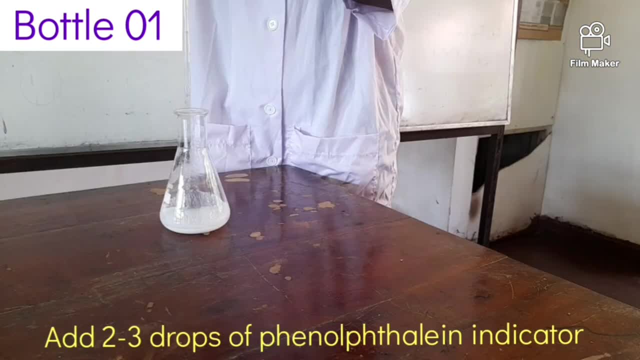 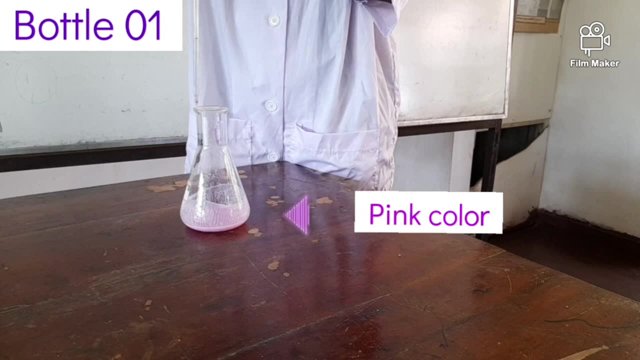 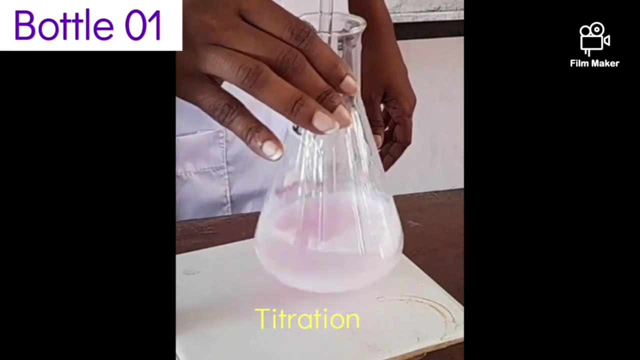 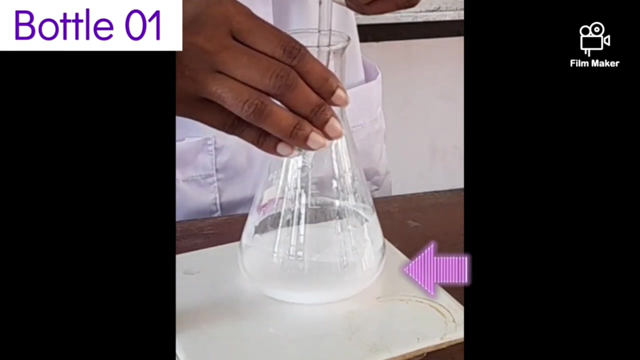 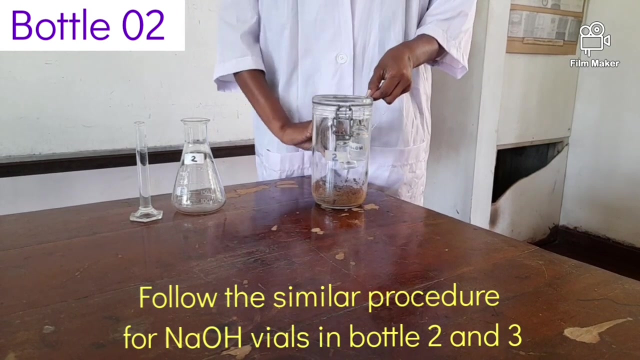 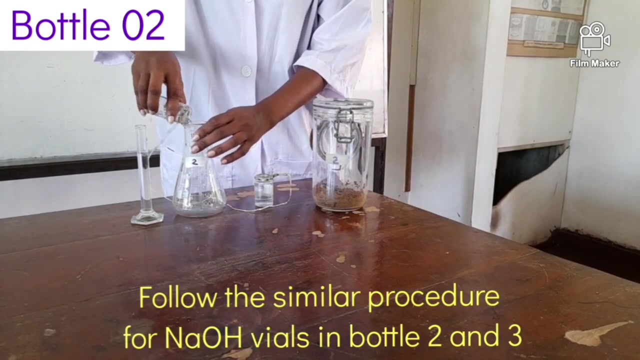 You can see the white colour precipitation. Then add 2-3 drops of phenolphthalein indicator and titrate the solution against 0.5 m HCl solution until you observe the colour change. You have to follow the exact similar procedure for the sodium hydroxide vials in the samples named as 2 and 3.. 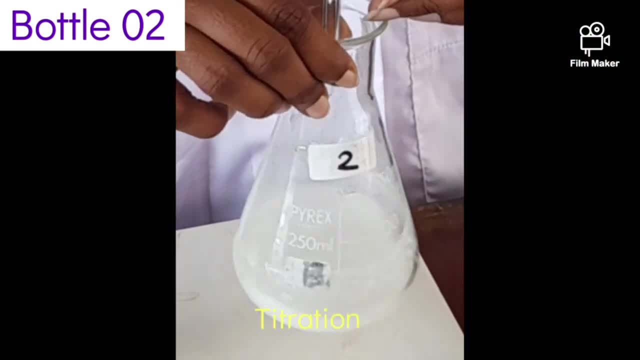 Nowイ dauid HCl and the соответing 1-mol sodium hydroxide vials into 2.5 m diluted water or 0.5 m HCl solution and fill the bottle with 0.5 m HCl solution. 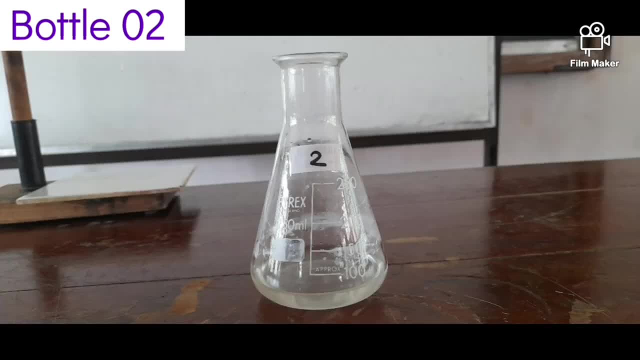 This smoke-free solution to dilute water reaches up to 20 mg per litre per year. Let's see if it can reach to 20 mg per litre. Here is the result for the sodium hydroxide vial. You see, the refractive temperature of the boiling water is about 22.5-23°C, so it is almost 22.5°C. 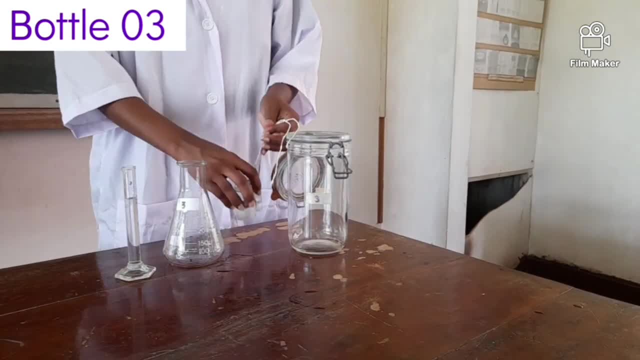 but the temperature of the boiling water is about 24.5°C. The twoißtated temperature of the boiling water is about 20°C, The temperature is about 8°C and ginger's temperature is about 40°C. You see the concentration of sodium hydroxide and the concentration of calcium hydroxide in the water. 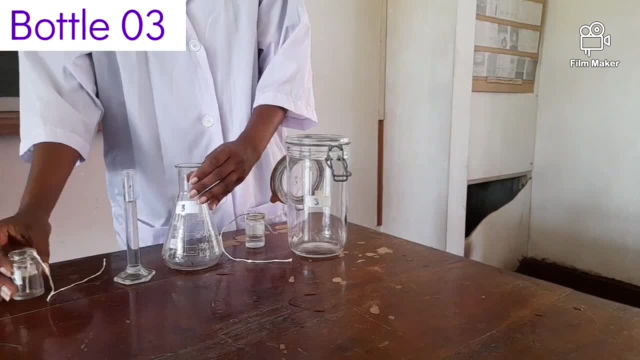 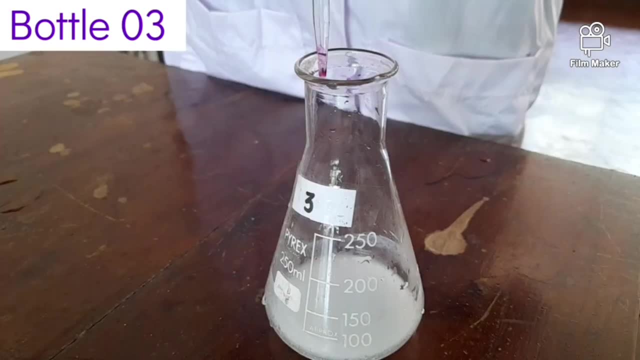 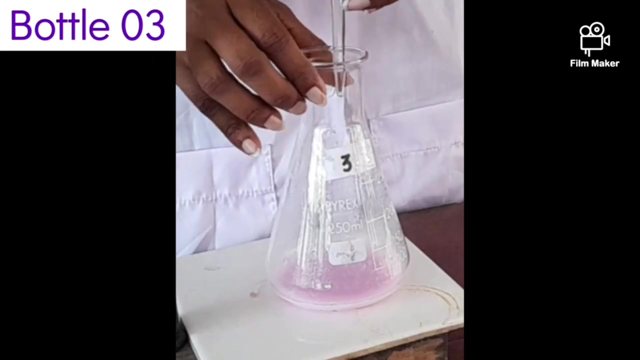 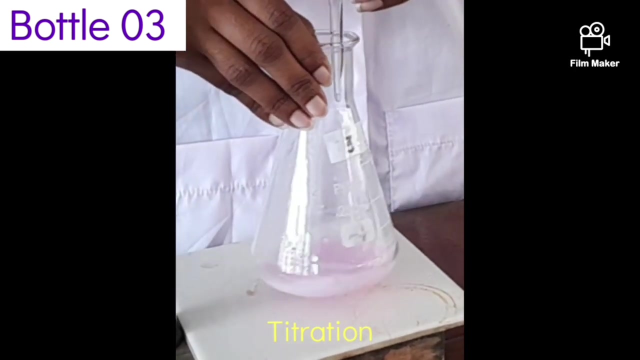 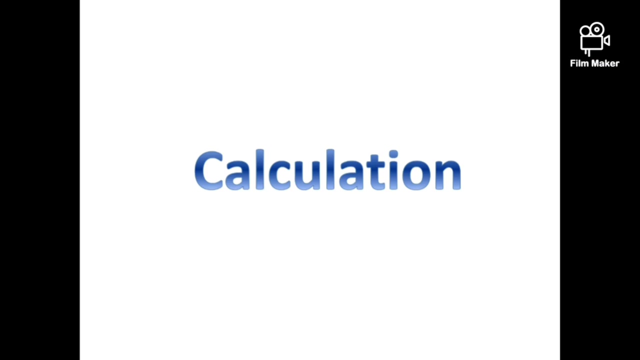 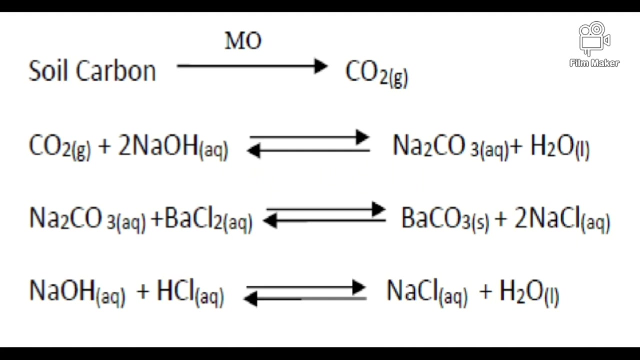 and how it is running Calculations. Due to the microbial respiration soil, carbon oxidized into carbon dioxide, which is reacted with sodium hydroxide in the vials by resulting sodium carbonate and water. After adding barium chloride, it converts into barium carbonate precipitate. 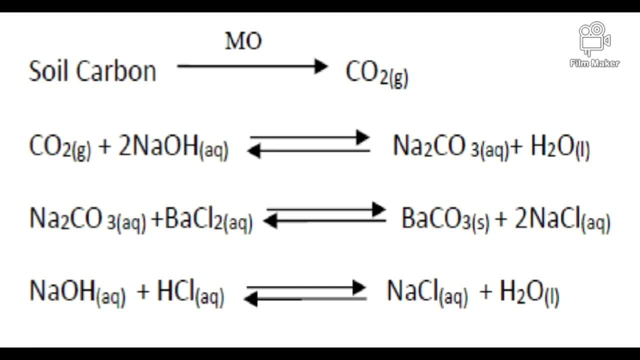 Then remaining sodium hydroxide could be determined by a backpite pressure Against 0.5 m HCl solution with the presence of phenolphthalein indicator, until observed a color change from pink to colorless. Since the concentrations and volumes of sodium hydroxide and hydrochloric acid are known, 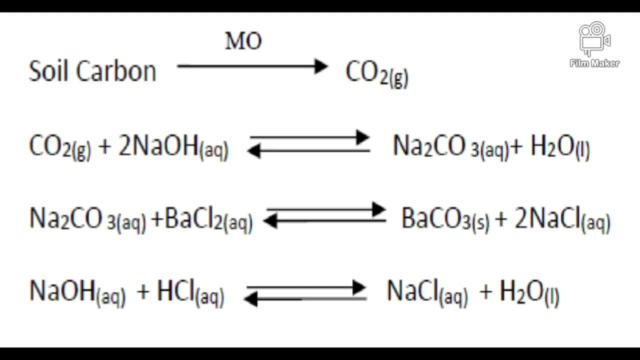 we will be able to calculate the number of moles of carbon dioxide released from the soil sample by using the stoichiometry. As the final conclusion, please refer below slides for further calculations.